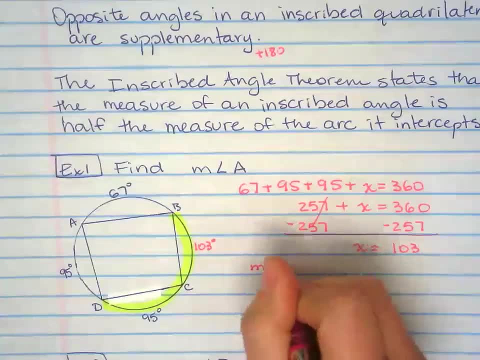 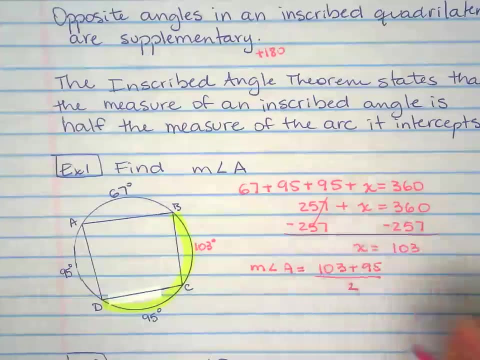 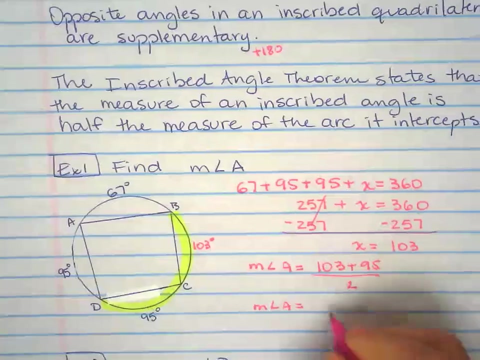 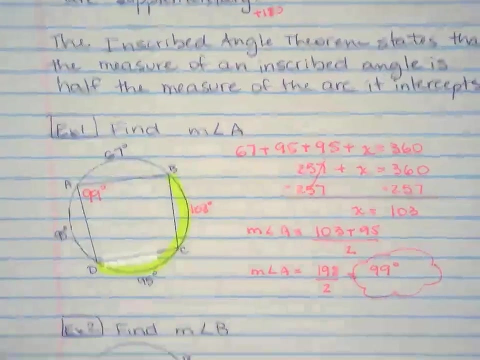 So if I know that, angle measure A is 103 plus 95.. Divide by 2.. Here I have 198.. Divide by 2. That will give me 99 degrees for this angle. right here More. So we need to find angle measure B. 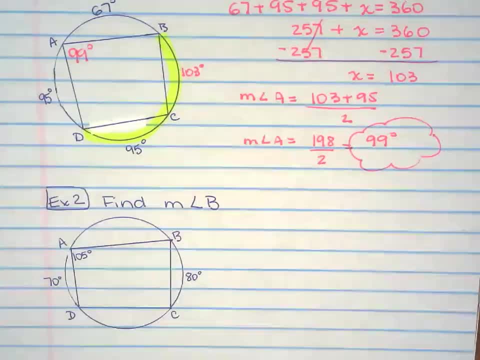 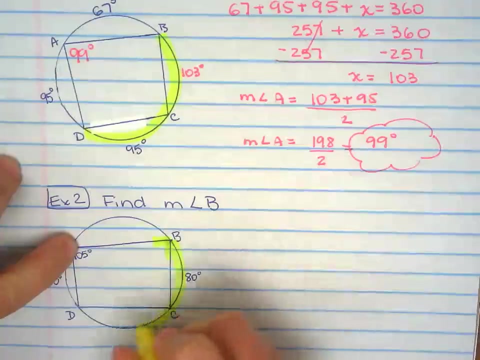 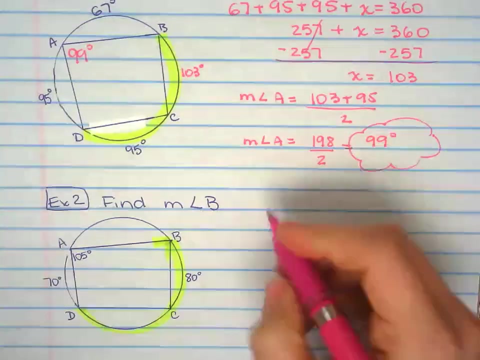 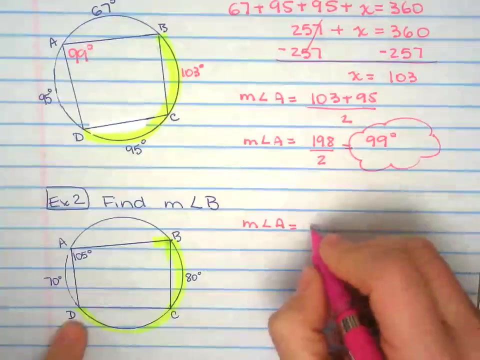 Okay, For this guy right here. So by the inscribed angle theorem, I know 105 is half of this arc right there And you're like, huh, how is that going to help me? Well, If I know that this is half of what the arc BCD is? 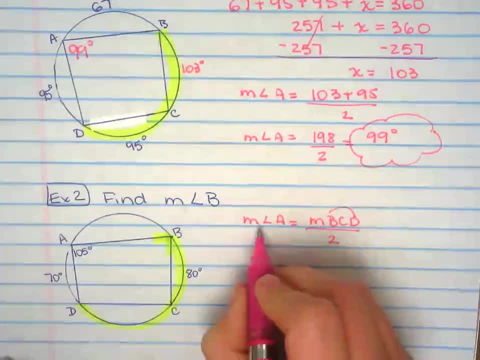 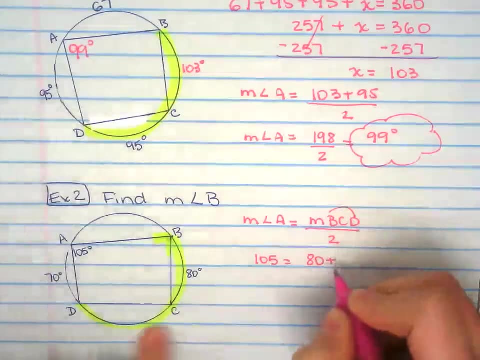 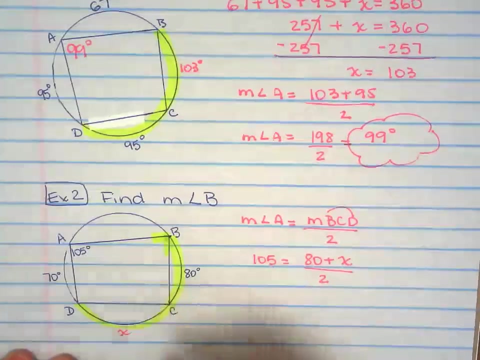 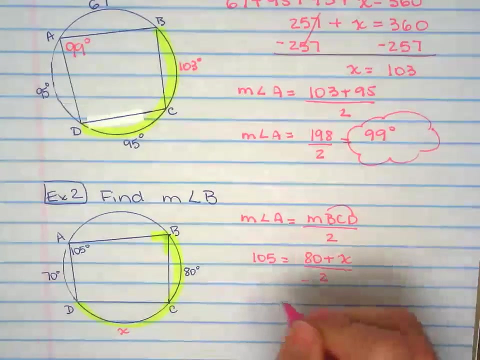 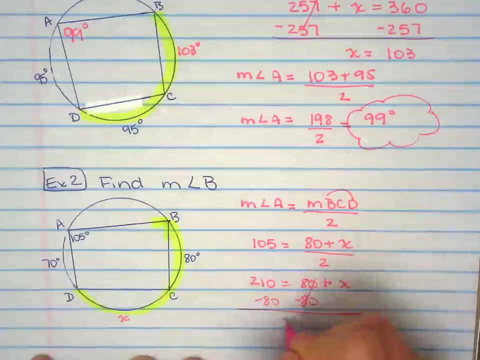 I have A, I have BC, I don't have CD. I don't have CD, So I'm going to find this guy first. Multiply by 2. Minus 80 from both sides, So I have X is 130.. 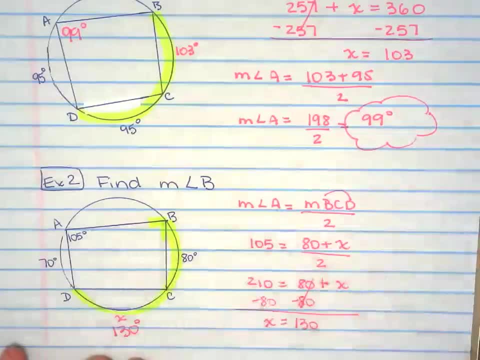 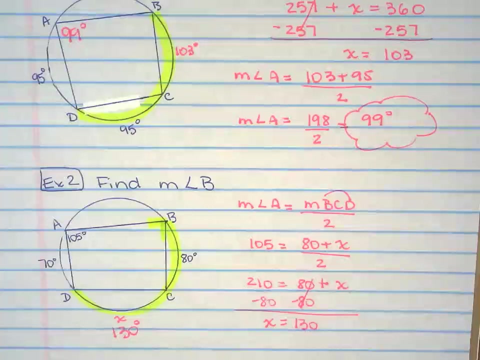 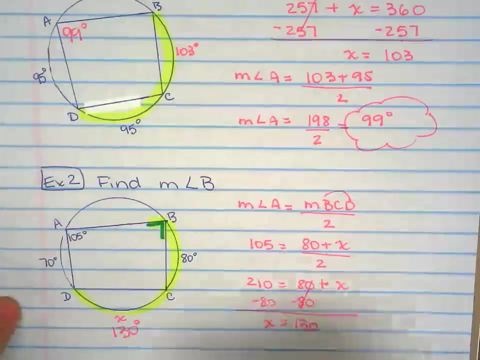 So this arc X, So this arc X is 130.. Now it's easy, because now that I have the arc, I have this guy and I have this guy, I'm going to use a different color. So if I'm looking for angle measure B, I know